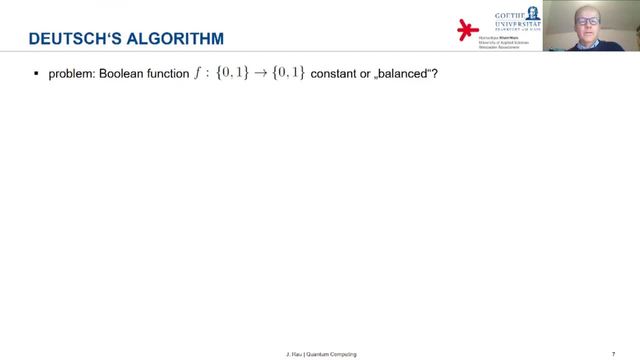 They map an input bit string- In this case it's just a single bit- with possible values 0 and 1- to an output bit with possible values 0 and 1.. And the question is whether this Boolean function is true, Or is it just a constant, meaning that f of 0 has the same value as f of 1.. 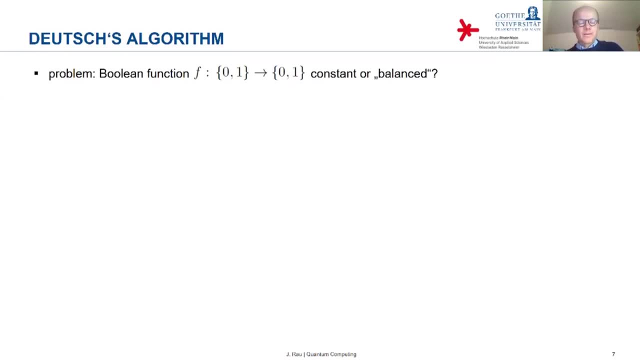 Or if the two values are different, the possible values of the function 0 and 1, they both occur. So once you have the value 0,, once you have the value 1.. And then the function is balanced. So both possible values of the function. 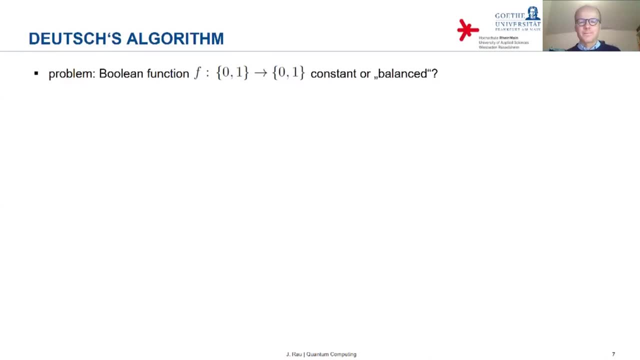 Occur once. Classically, what would you do If you just evaluate the function for the two possible values of the input And then you compare the outcomes, And if they are equal then the function is constant, And if they are different, then the function is balanced? 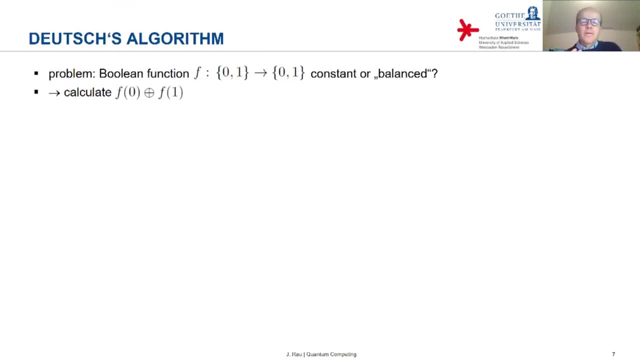 So answering this question is equivalent to calculating the sum of f of 0 and f of 1, modular too, Because if, if the function is constant, say the function is zero for both possible values of the argument, Then f of 0 is zero and f of 1 is zero. 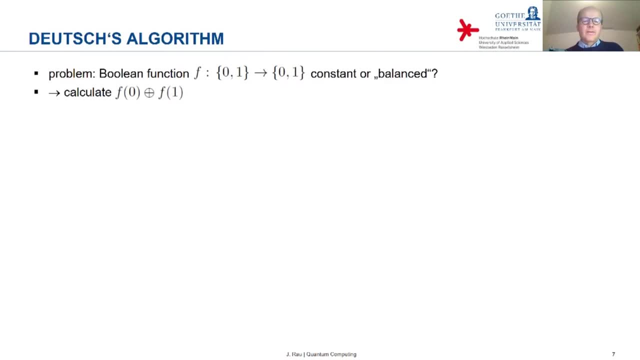 And the sum is also zero. If the constant value of the function is equal to 1,, then this sum is 1 plus 1 is 2, modulo 2 is also 0. So if the function is constant, then this sum mod 2 is 0. 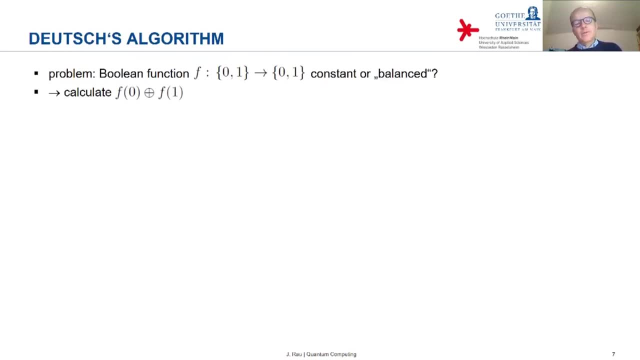 And if the function is balanced, so if the two values are different, then you have 0 plus 1 and this is 1.. So one way of answering the question is to calculate this sum. And if the sum is 0, then the function is constant. 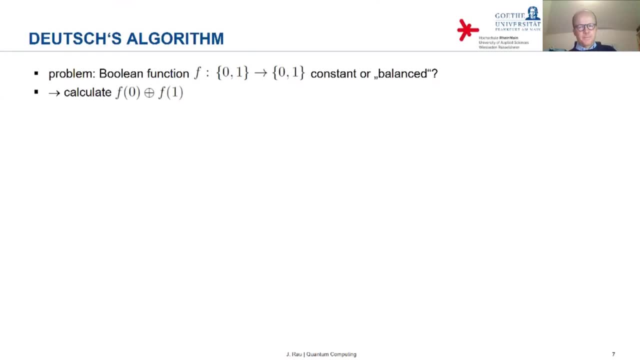 If the sum is 1,, then the function is balanced. Now David Deutsch developed a little circuit which performs that calculation, And it makes use of a particular kind of gauge, A gauge called an oracle. You can think of an oracle as in Greek mythology. 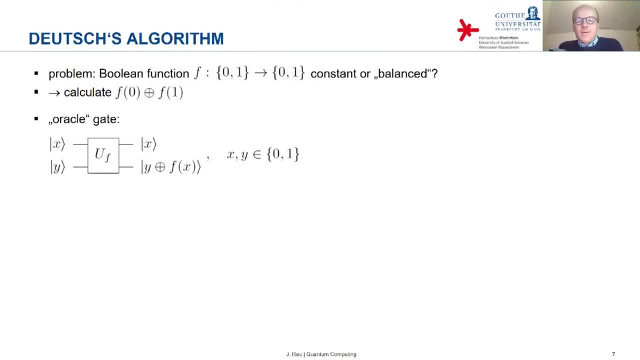 You go to an oracle when you have a question And you ask the oracle for an answer. And here you have a question about the value of the function and the oracle gives you the answer. Here is precisely what the oracle does. You have two. it's a two qubit gate. 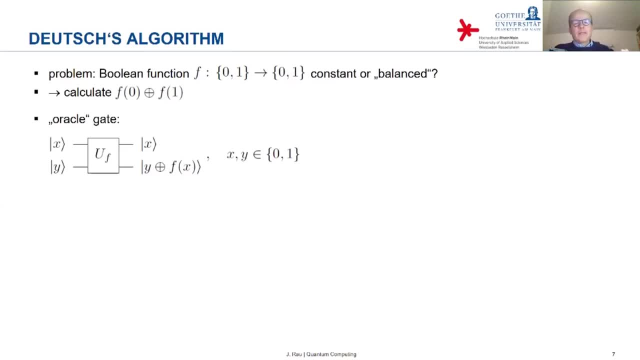 When the two input qubits are in basis states x and y. So x and y are either 0 or 1. Then the upper qubit exits in the same state. So it's a bit like a control qubit in the CNOT. 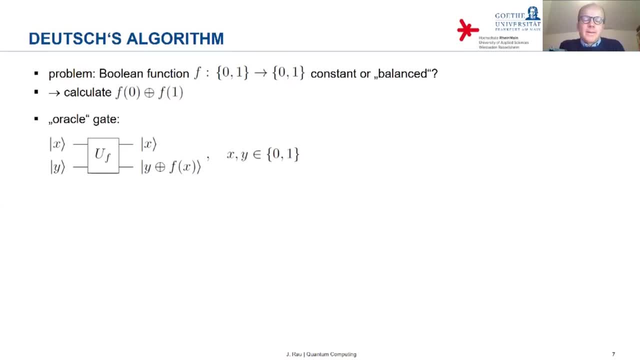 So its basis state does not change, Whereas the lower qubit may change. So if f is 0, then the lower qubit is unchanged, But if f is 1,, the lower qubit- the basis state of the lower qubit is flipped. 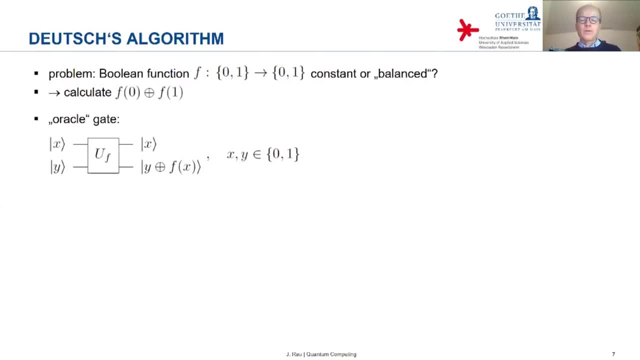 Then you apply a plus 1 mod 2, which is equivalent to a flip. We had that earlier. So, in short, the oracle, when basis states are coming in, the oracle leaves the upper qubit unchanged, The basis state unchanged, And the lower qubit- the basis state, is flipped. 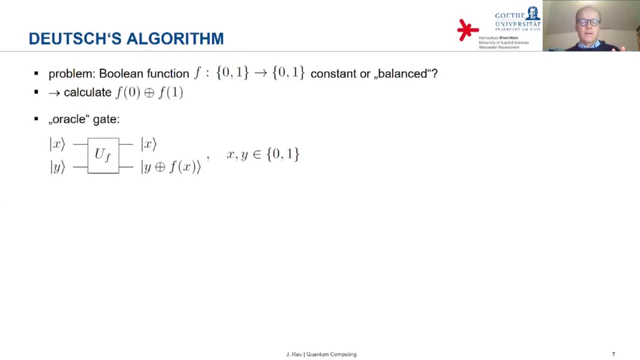 If, and only if, f is 1.. Now, this may look like a somewhat weird way of calling the function, But that's a way of inquiring about the function. Now, the reason it takes this peculiar form is that, of course, in order to implement such a gate, this must correspond to a unitary transformation. 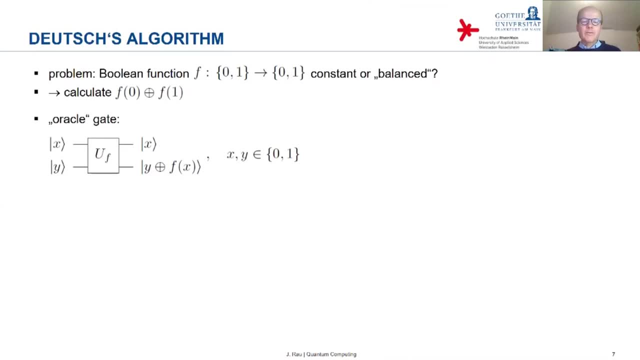 So there must exist a unitary transformation which does precisely that. And here I show you, in the standard basis, the matrix representation of that gate. First of all, you can convince yourself that it does precisely what the graphic shows. It has this block diagonal form. 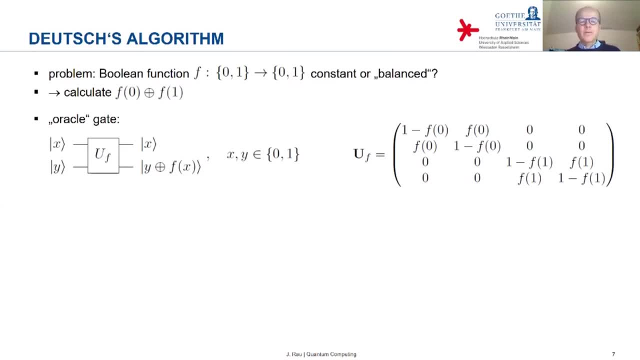 The block diagonal form in the standard basis, first of all, shows you that it doesn't change the state of the first qubit, Only the state of the second qubit In the upper left 2x2 matrix. this is the transformation applied to the lower qubit when the upper qubit is in the basis state 0.. 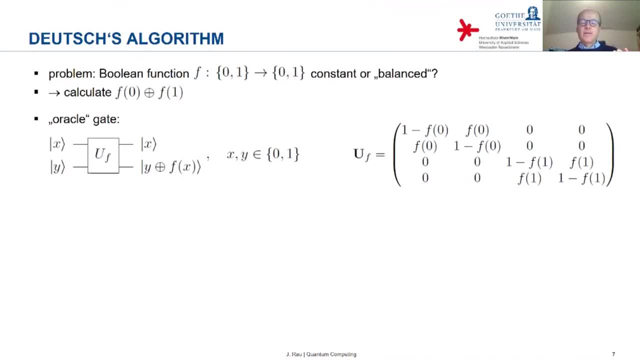 And so when x is equal to 0. And then you see, if f is 0, then in the upper left you just have the 2x2 unit matrix, And this means that the state of the lower qubit doesn't change. 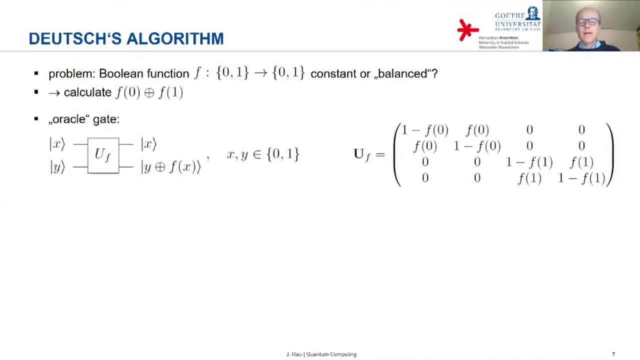 As is shown also in the circuit. If, on the other hand, f is 1,, then the 2x2 matrix in the upper left corner is the Pauli x. You have 0 on the diagonal and 1 on the off diagonal. 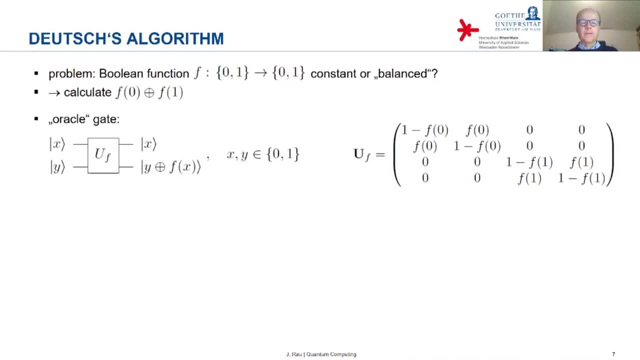 So this is the Pauli x, and the Pauli x does a flip. So then the lower qubit state flips as is shown in the circuit, And you can make the same argument for the bottom right 2x2 matrix, That if f 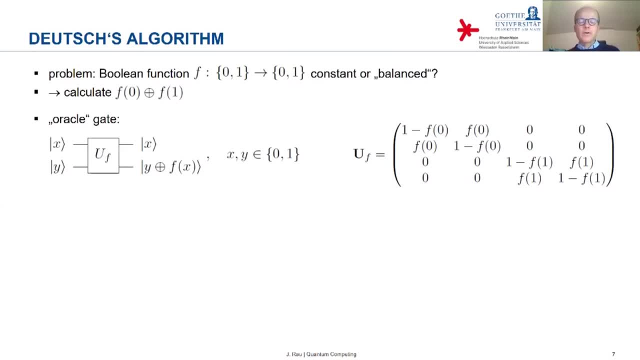 so this shows you how the lower qubit is transformed when the upper qubit is in the basis state 1. So when x is equal to 1.. And then you see, if f so f is f is equal to 0, nothing happens. 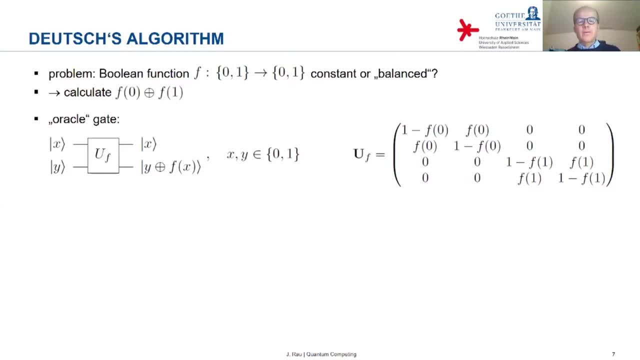 If f is 1,, then again you have the Pauli x in the lower right and you have a flip. So this matrix does exactly what's shown in the circuit, And then we just have to verify that the matrix is unitary. Well, it is real. 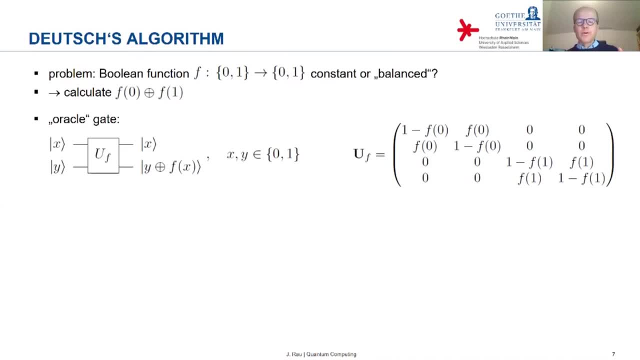 It is symmetric, So it is Hermitian, And the square of the matrix gives the unit matrix, And so in the upper left and in the bottom right, depending on the values of the function, you have either the unit matrix or the Pauli x. 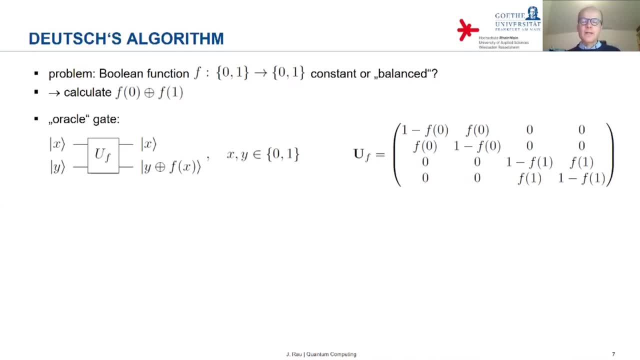 But in either case, the square of the unit matrix and the square of the Pauli matrix are the unit matrix. So, regardless of the value of the function, the square of this unitary matrix is the unit matrix. Yeah, So it's Hermitian. 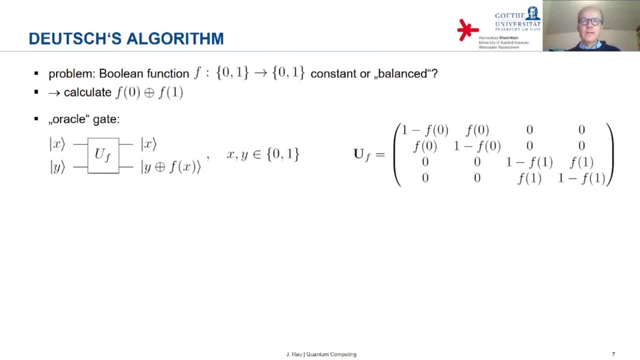 The square is equal to the unit matrix And this means that U U dagger equals U squared. because U dagger is equal to U equals the unit matrix, So U U dagger's unit matrix- that's by definition, shows that U is unitary. 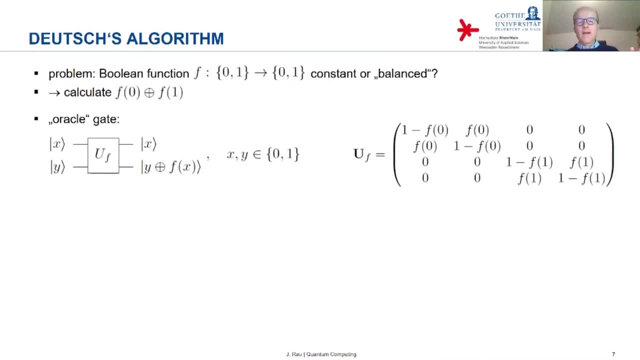 Okay, So we have this oracle wherever it comes from, But conceptually it exists and it represents. it's a unitary transformation, It's a possible gate. And now Deutsch circuit proceeds as follows: You have two input qubits, one in the basis state, zero. 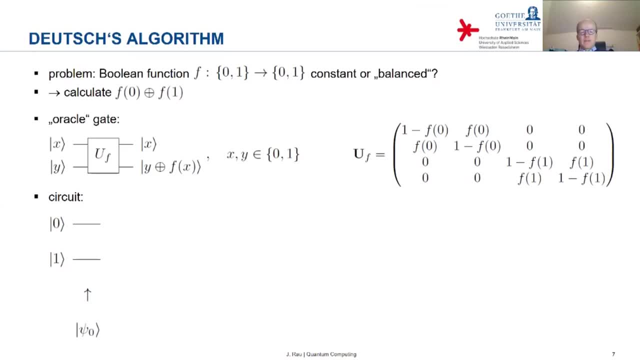 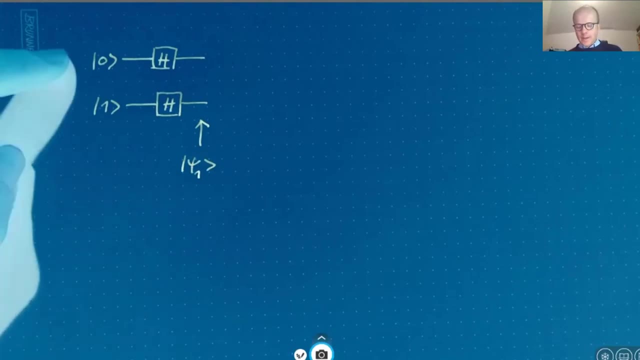 and the other in the basis state one. The first thing that happens is that you apply to both qubits a Hadamard gate. The Hadamard gate applied to the first qubit, transforms the basis state zero to a plus state, and the Hadamard gate below transforms the basis state one to a minus state. 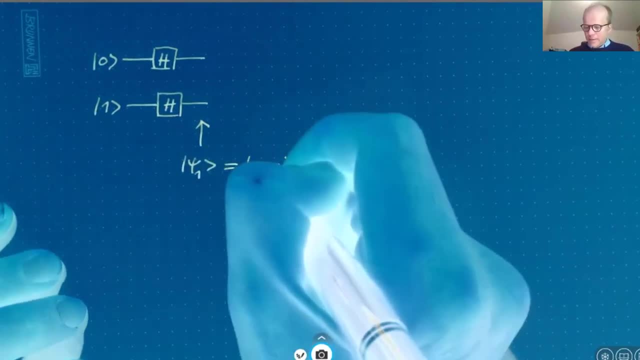 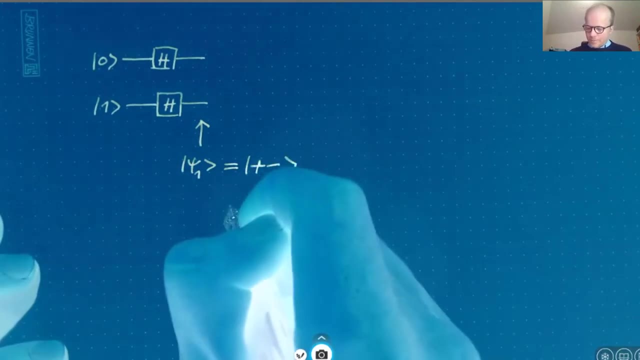 So psi one, that's the state for both qubits, that's the state plus, minus. Or if I write out explicitly the plus state, then it's zero plus one over square root of two, or the first qubit tensor minus In the step after that. 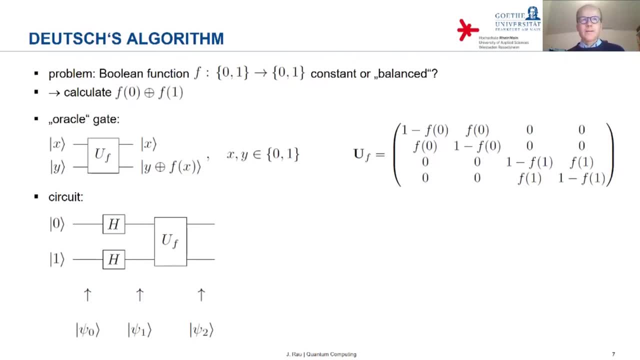 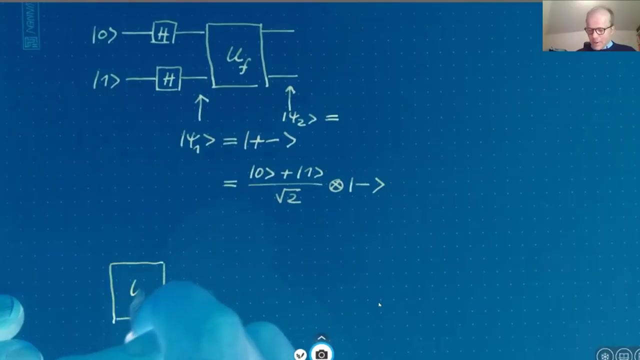 these two qubits enter the oracle. So essentially we make a function, call Yeah, One query about the values, the value of the function. One little result on the side about the oracle. Imagine you have the two qubits going in, The first one in the basis state x. 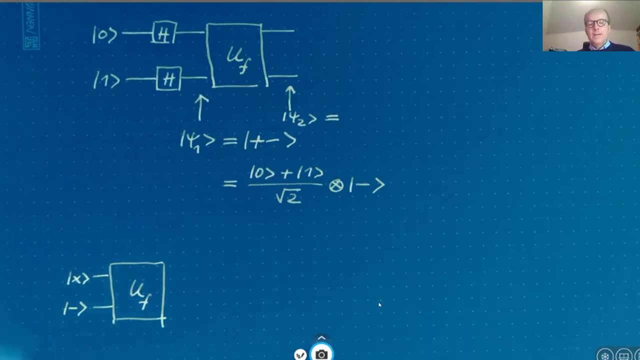 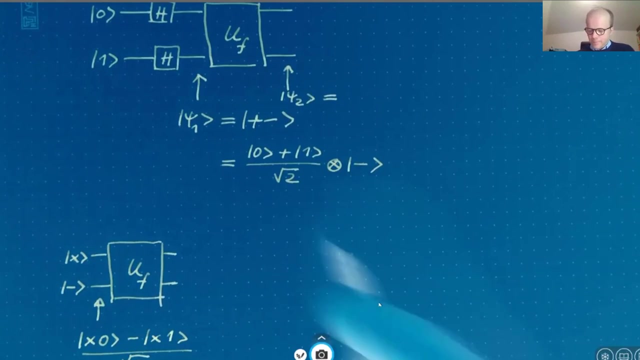 and the second one in the state minus, in the minus state, So not a basis state. Well, this state here, yeah, this can be written as zero minus one over square root of two. So this is the two qubit state going into the oracle. 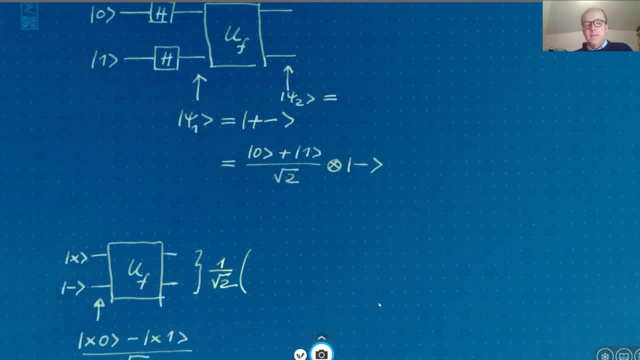 And what does the oracle do? Well, when you have basis states, then the coming in, then the first basis state is not changed. So the x zero is mapped to x. the x remains the first qubit remains in the same state. 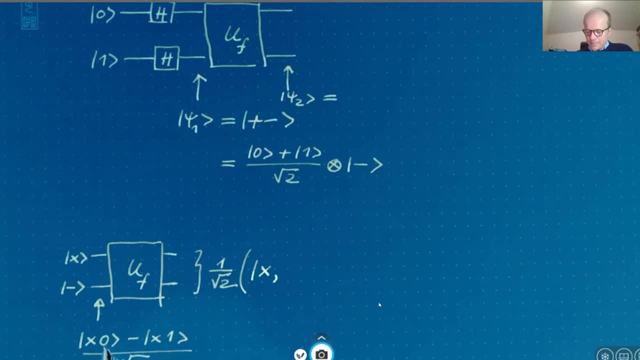 The state of the second qubit is changed depending on the value of the function evaluated on x- And remember that was it was an addition- plus the value of the function f plus f of x mod two. So we here we have in this case zero. 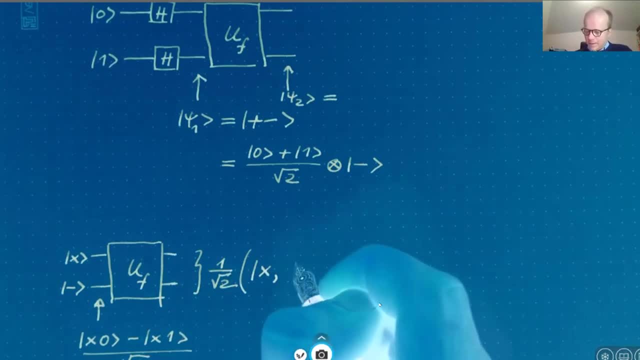 plus f of x And this this gives f of x. From this we subtract the oracle applied to x one. Again, the x is unchanged, And to the one we have to add the value of the function f of x mod two. So this, the one is: 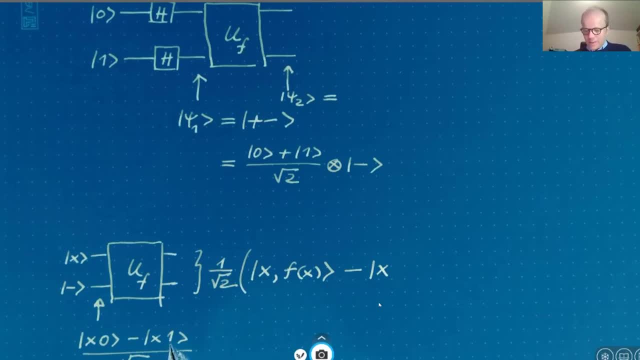 flipped if f of x is equal to one And it remains unchanged. if f of x is equal to zero, One way to write this is to say: this is one minus f of x. So if f of x is zero, then the state of the second qubit is still one. 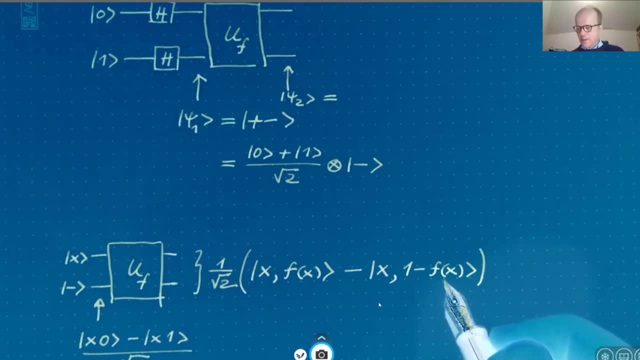 It's unchanged. If f of x is equal to one, then this is zero. So the state of the second qubit has flipped. So this is a way of writing the state after the oracle. Now there are two possibilities. f of x can be either zero. 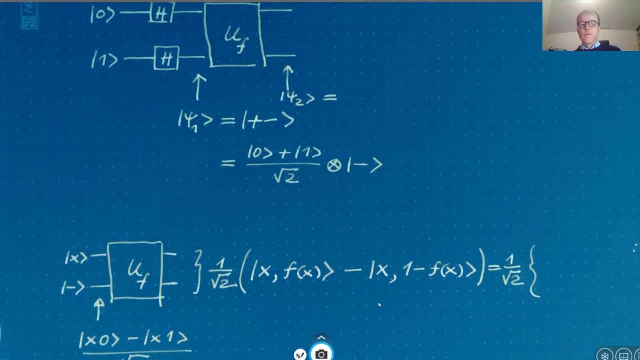 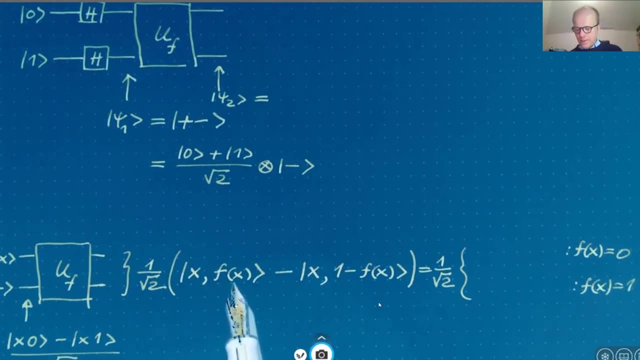 or it can be one. If f of x is zero, then the result here is x zero minus x one, And that's precisely the state. that is the state that went in. So that is, I could have done without the one over square root of two. 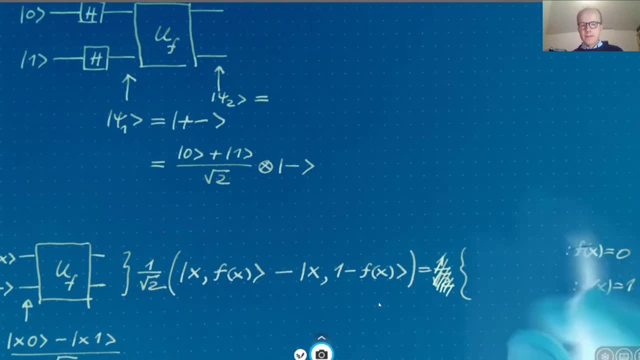 divided then by square root of two, This is precisely x minus. That's precisely the state that went in. If the value of the function f of x is equal to one, then we have x one minus x zero. That is equal to the input state. 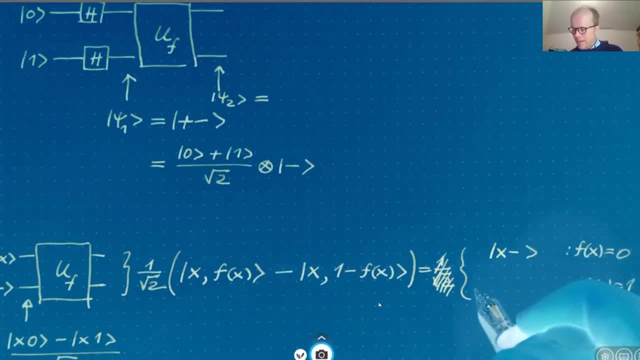 up to a sign. So that is minus, x, minus, And we can summarize this finding by writing the output state as minus one to the power f of x times x minus. What you see is that the, the two qubit state, x, zero, is an eigenstate of the oracle. 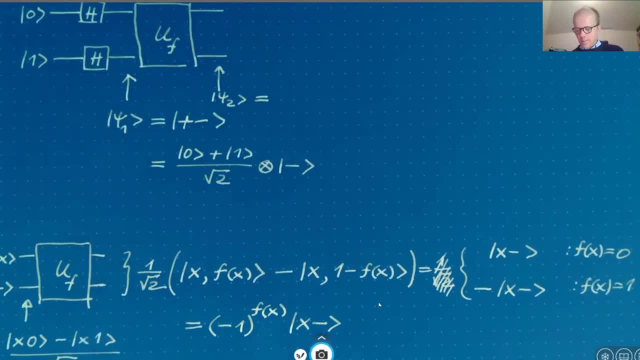 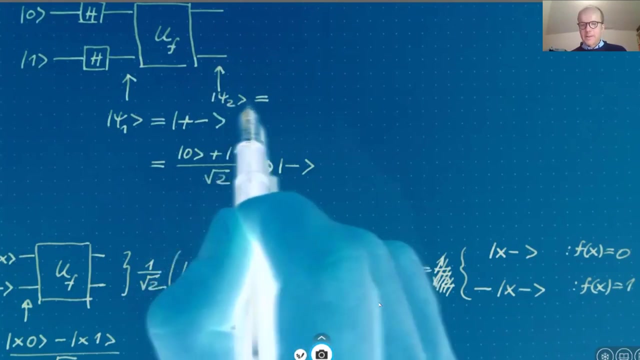 And the two possible eigenvalues are plus one and minus one, And whether you have plus or minus one depends on f of x. Okay, This result I would like to use to calculate this state here. after the oracle, Just before the oracle, we had this one, remember. 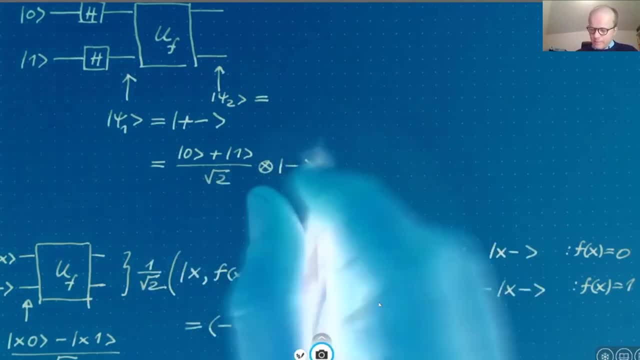 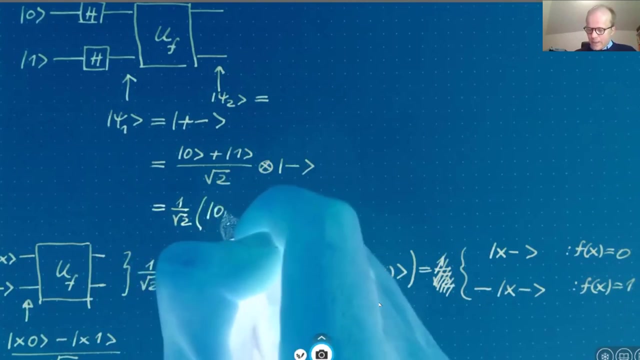 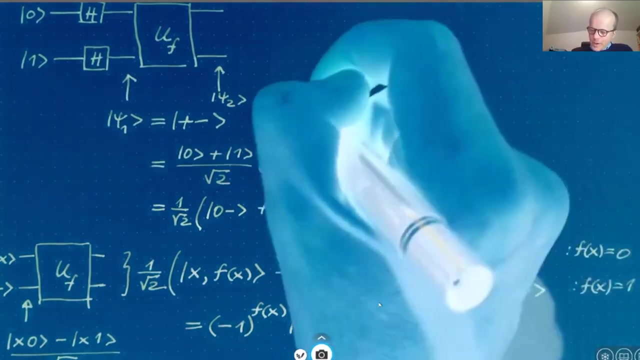 Yeah, And maybe let me pull it apart and say: this is one over square root of two, And then we have zero minus plus one minus Okay. Then we to this state here, we apply the oracle and we use the result down here And then we find: 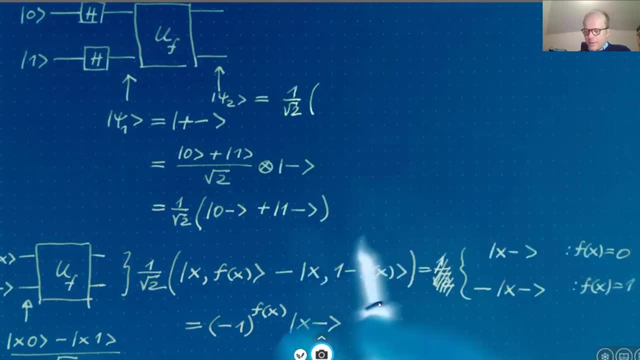 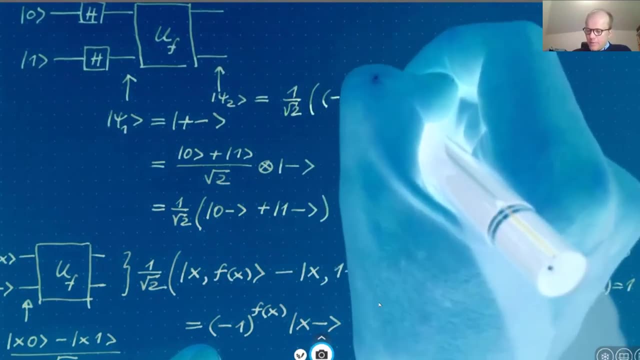 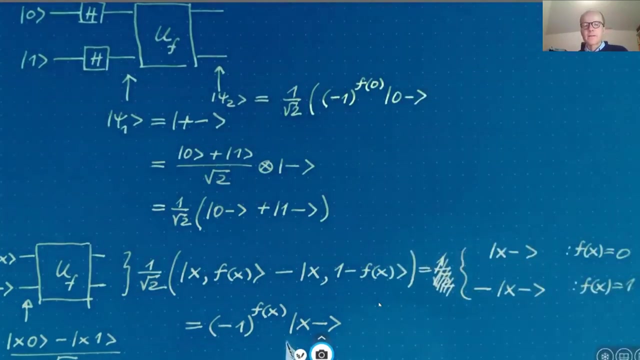 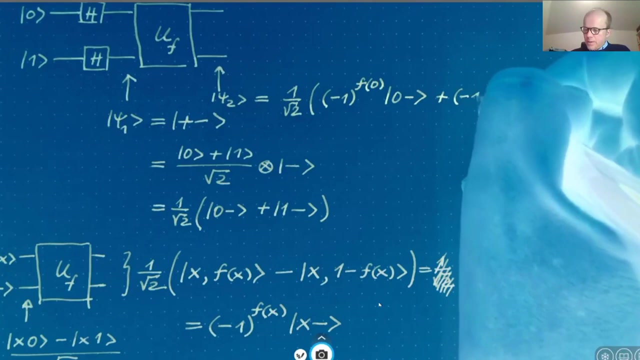 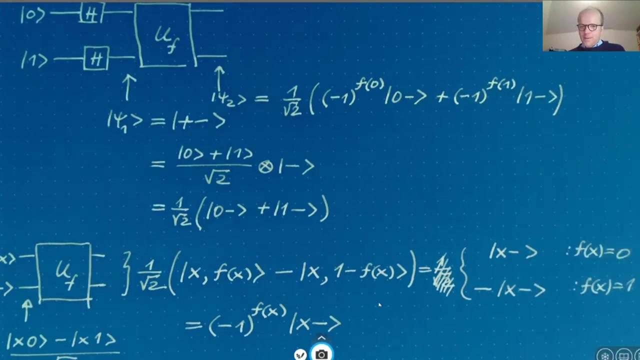 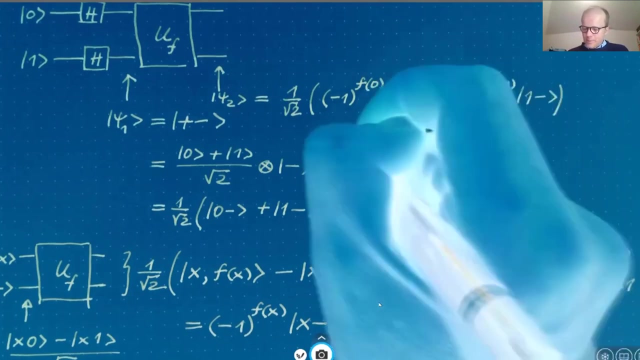 that the zero minus becomes minus one to the power f of zero times zero minus using this result down here. And the one minus becomes minus one to the power f of one one minus. Now let's consider two possible cases for the for the psi two: 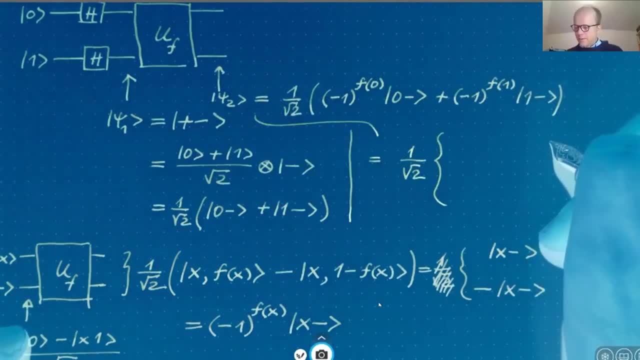 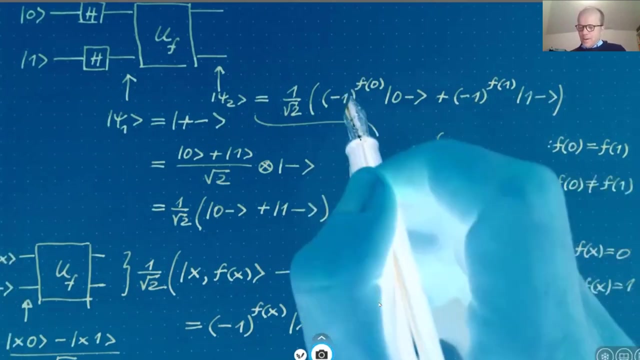 Depending on whether the function is constant or the function is balanced. Let's assume the function is constant, So f of zero is equal to f of one, In this case minus one to the power f of zero and minus one to the power f of one. 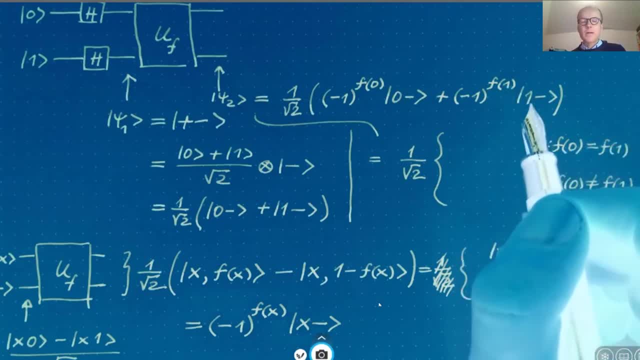 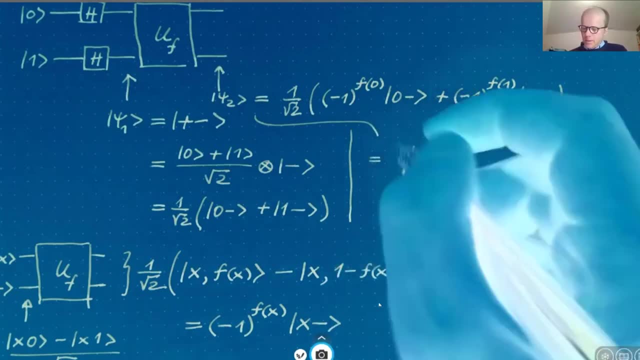 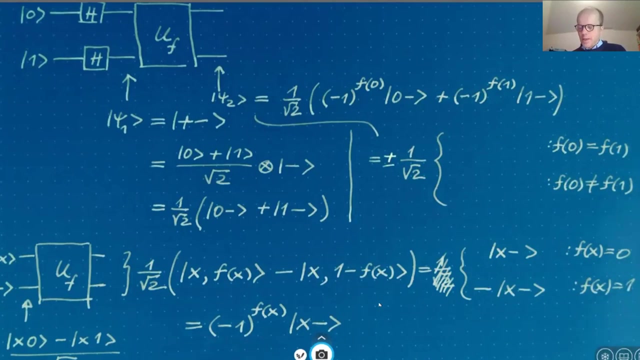 are equal And they are both either plus one or minus one. So up to an overall sign which I write in front of the prefactor here, up to an overall sign we have here: zero one, zero minus, plus one minus. So let me write it in this form: 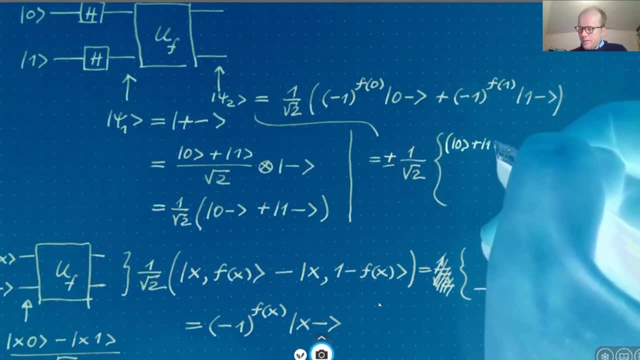 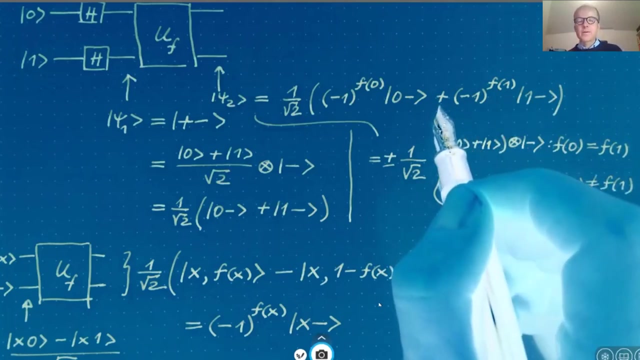 zero plus one tensor minus. If the two values are different, then we get here the minus one to the power f of zero and the minus one to the power f of one. they have opposite signs. So we get here a relative sign, minus. So again we can take out: 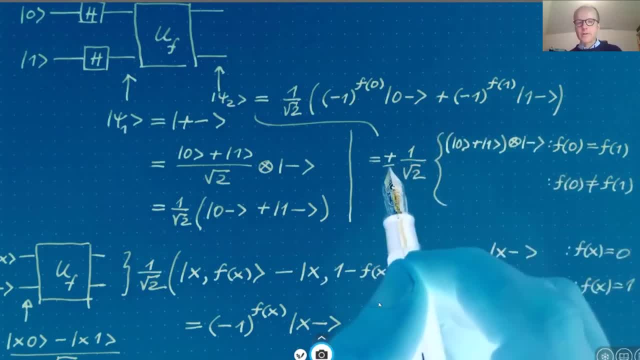 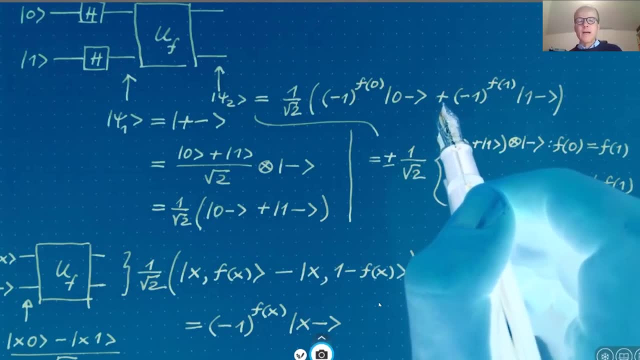 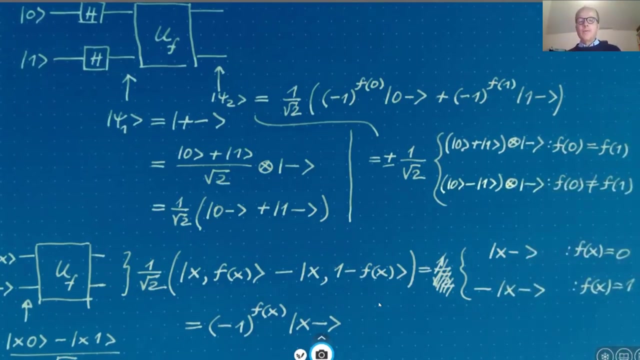 sort of a global sign to the front And we have in between here we have a relative sign, minus. So then we get here: zero minus one tensor minus. So these are the two possibilities, depending on whether the function is constant or balanced. We can also, actually we can- write it. 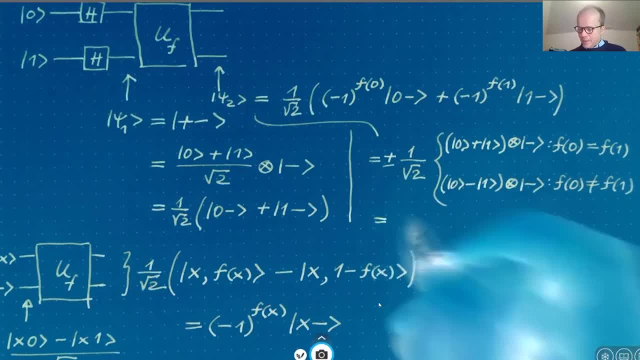 even shorter. This is plus or minus. And then the combination zero plus one divided by square root of two, that's precisely the state plus. So then we have plus, minus. and zero minus one over square root of two, that's the state minus. So then we have minus minus. 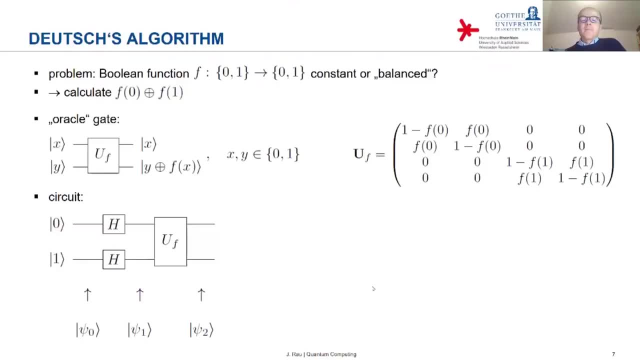 Okay, let's get back to our circuit. So, in short, what we found in our calculation? the psi two is up to a global sign, which doesn't matter. It's the state plus- minus if the function is constant, and it's the state minus- minus if the function is balanced. 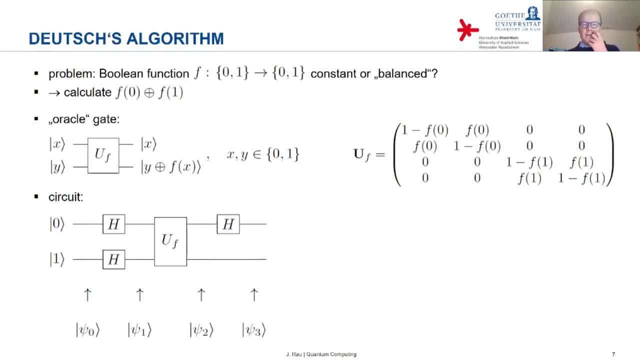 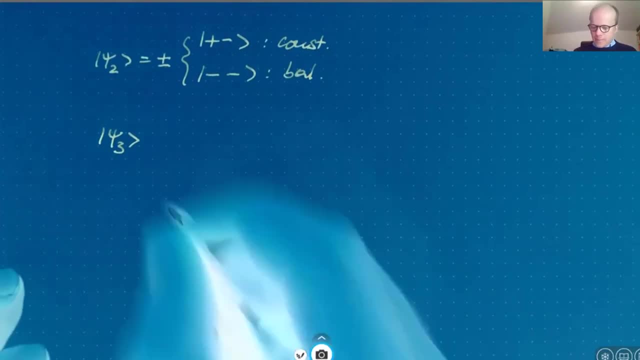 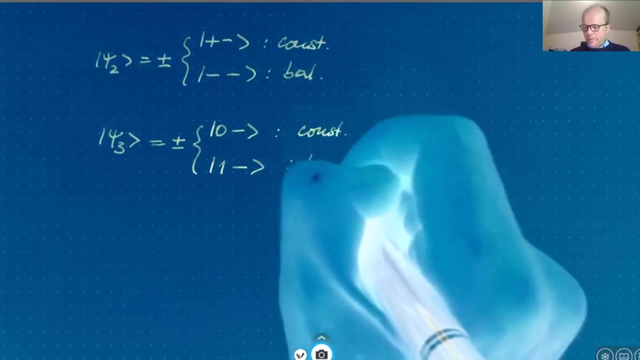 Then we apply a Hadamard gate, but to the first qubit only. The Hadamard gate transforms a plus state to a basis state zero and a minus state to basis state one. So we have the state psi three after this Hadamard gate. 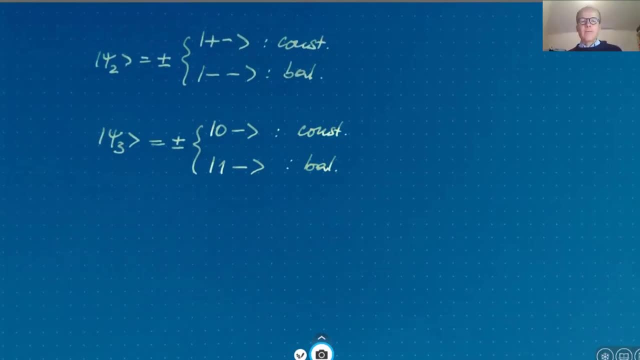 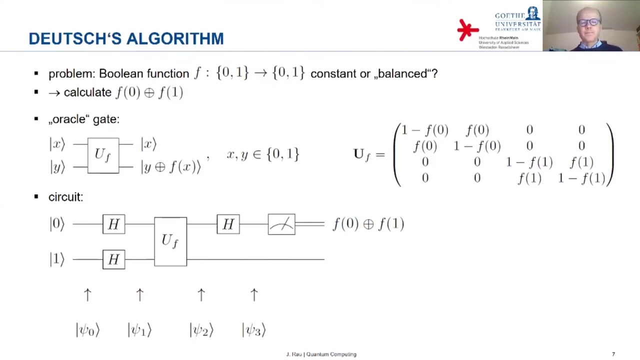 is either zero minus if the function is constant, or one minus if the function is balanced. And then in the final step we perform a measurement only on the first qubit in the standard basis. Now we learned that from our calculation of the state psi three. 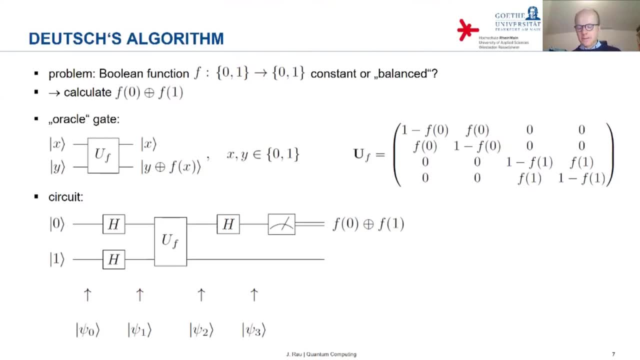 just before the measurement, that the first qubit is in the basis state zero if the function is constant and the first qubit is in the basis state one if the function is balanced. So when we perform a measurement and we find the outcome corresponding to basis state zero, 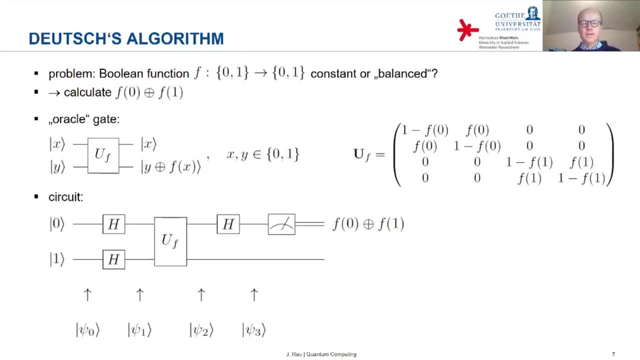 then we know the function must be constant. And if we find the outcome corresponding to basis state one, so if we find the outcome equal to one, then we know the function must be balanced. And that's the two possible outcomes: zero or one. that's precisely the 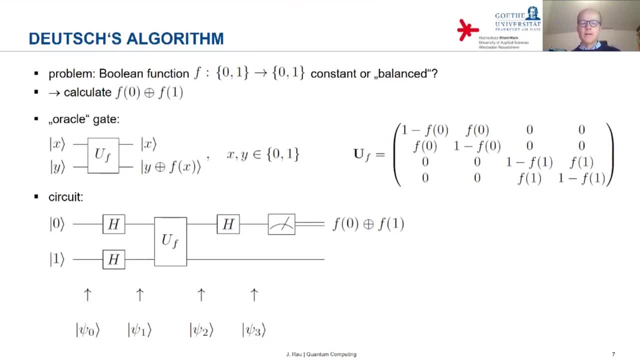 sum that we discussed before, f zero plus plus f one mod two, where we said: if the sum is zero, then the function is constant, if the sum is one, then the function is balanced. So this is the end of the circuit, and let's reflect on what. 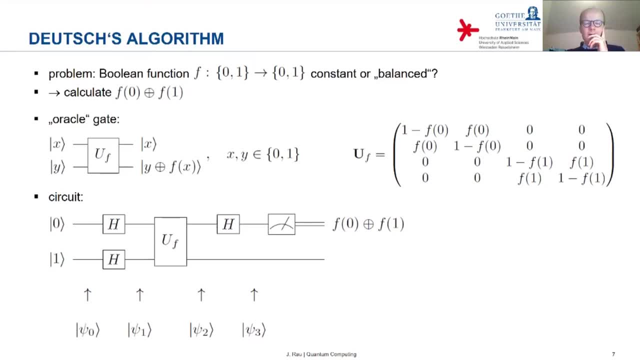 we have done. I mean, it looks at first like a a weird way of checking whether the function is constant or balanced. What's the attraction and what's the peculiar feature of the circuit compared to the classical algorithm which would just call the function for each value of the argument? 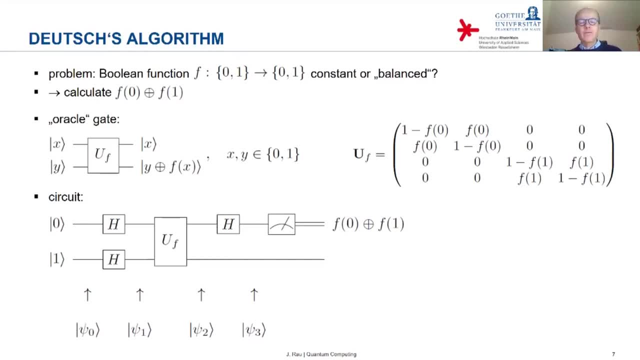 so we would call the function twice- f of zero and f of one- and just compare. and if they are equal, then it's constant, if not, then it's balanced. What's interesting about this circuit is the fact that here the function has been called only once.